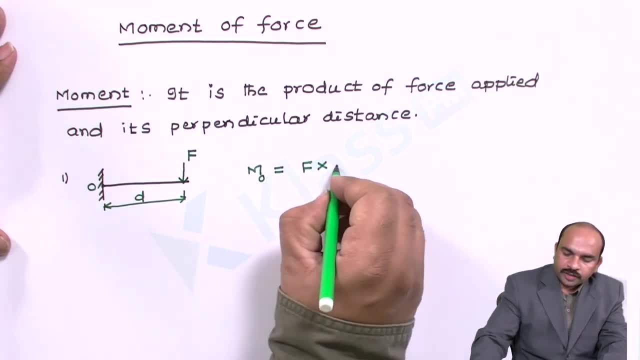 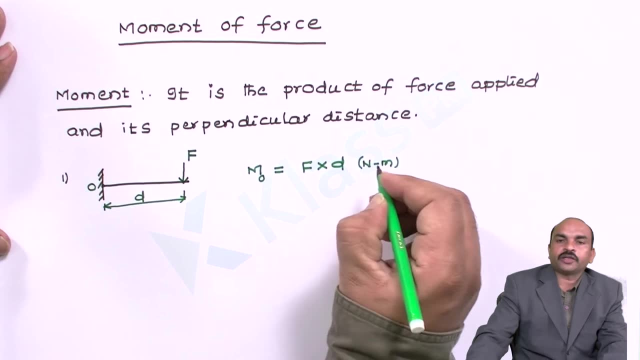 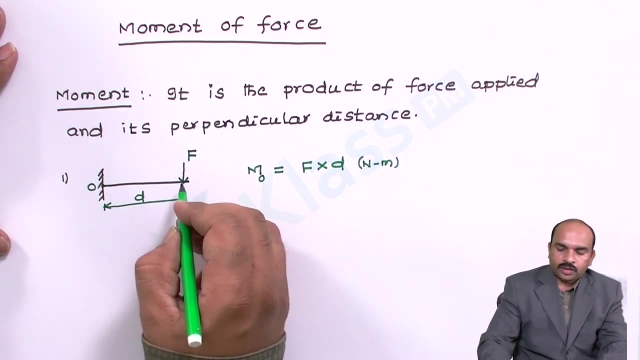 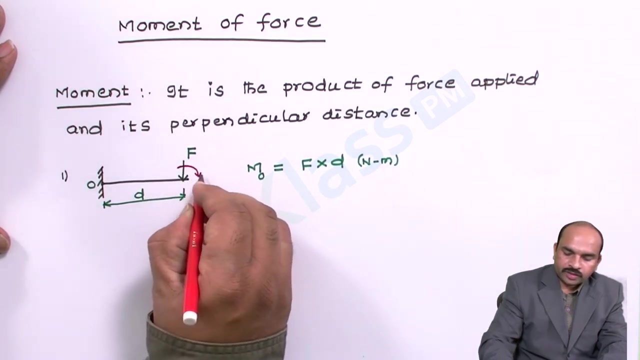 applied into its perpendicular distance D. We know force unit is Newton, distance unit is meter, So the units for the moment are Newton meters. Now, in this case, because of multiplication of this force, so it will rotate in clockwise, so the body will rotate in clockwise, so we say this as a clockwise moment. 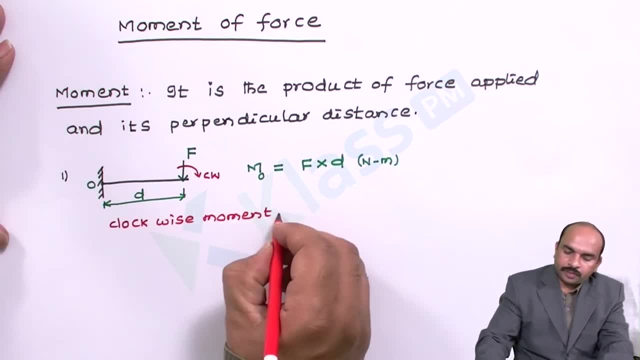 So clockwise moment we are taking as a positive sign And we solve the problem. Now the second type of the moment is anticlockwise moment. So let us see the anticlockwise moment. Let a force F applied in the upward direction. let us say its distance is D perpendicular. 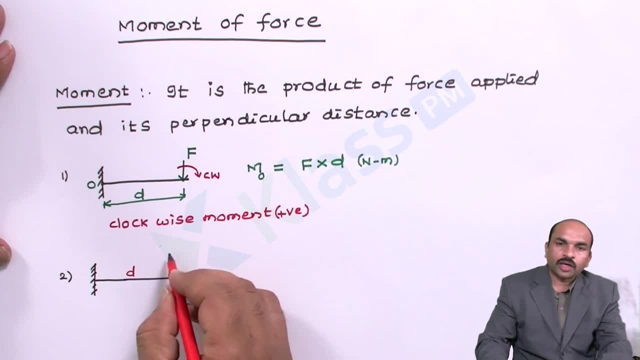 distance is D, then the body will move in the upward direction. So it creates an anticlockwise moment or counterclockwise moment. Now the moment with respect to O is equal to force into its perpendicular distance D, and anticlockwise moment we will take as a negative. 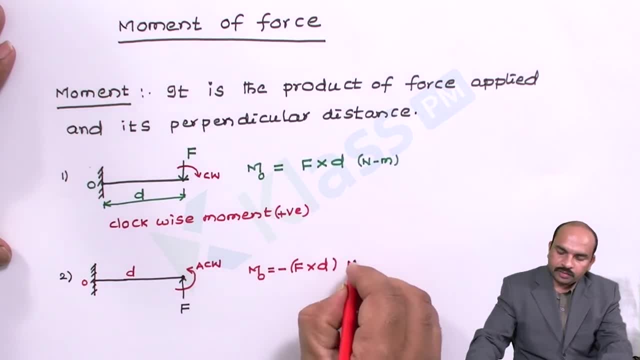 So that is the moment. Now the units are same Newton meter and it is a counterclockwise moment or anticlockwise moment. So these are the two types of moments are available and this is the moment top. of course we are talking about moment top. 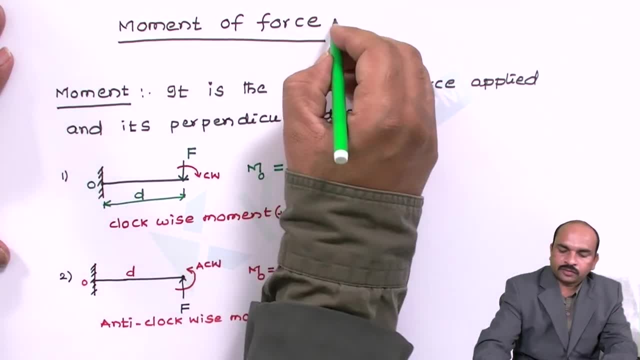 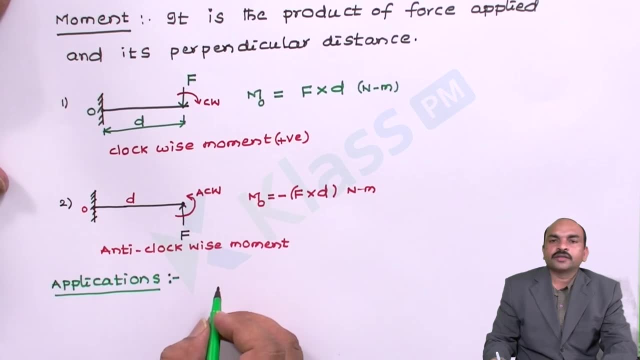 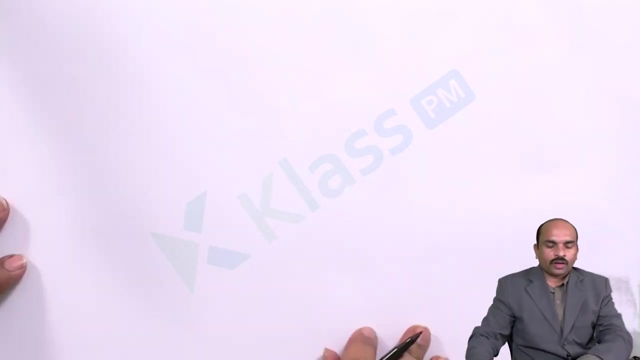 Now coming to its applications, moment applications. so moment is useful to protect any body. What is the purpose of moment? The application of moment, or the purpose of moment, Moment is to protect, is to protect any object. Now let us take some example, problems of moment. 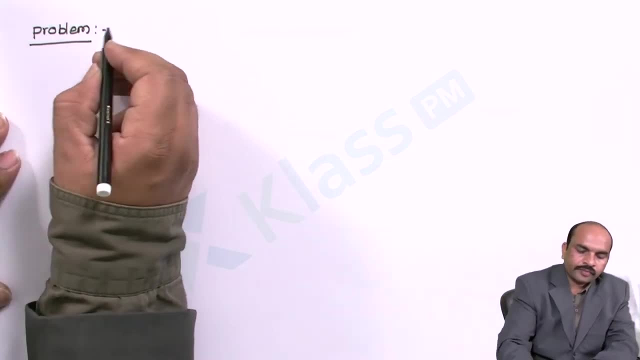 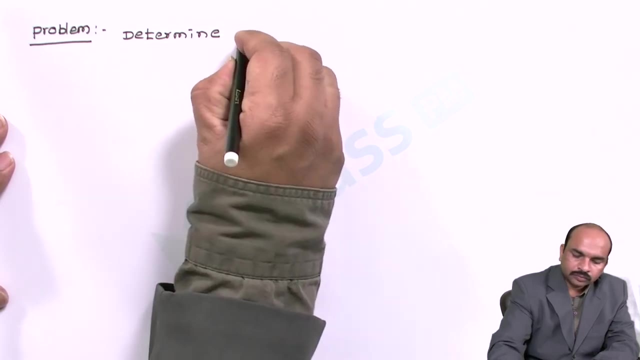 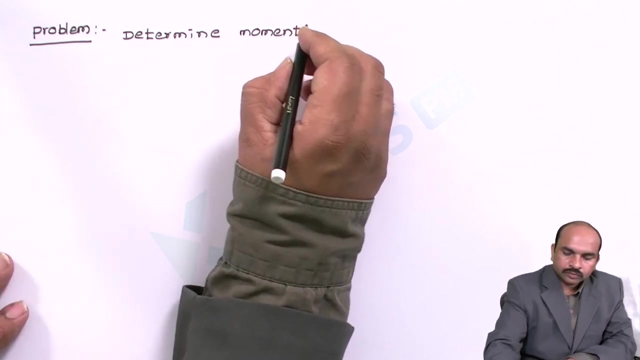 Moment is the moment égal or orthogonal to moment. Moment is determine the moment of moment. Moment of moment is necessary for sense of it or new design. Dear friends, if you do not manage the moment, you get hit by two så far situation and any 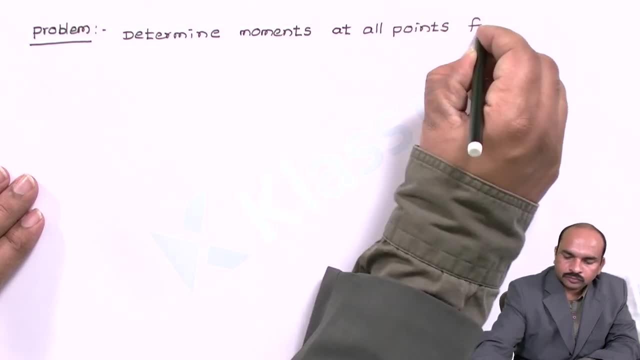 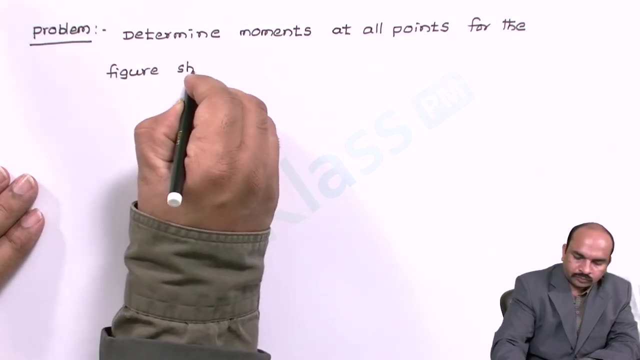 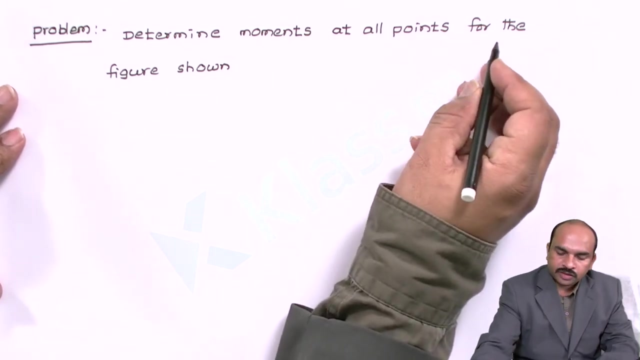 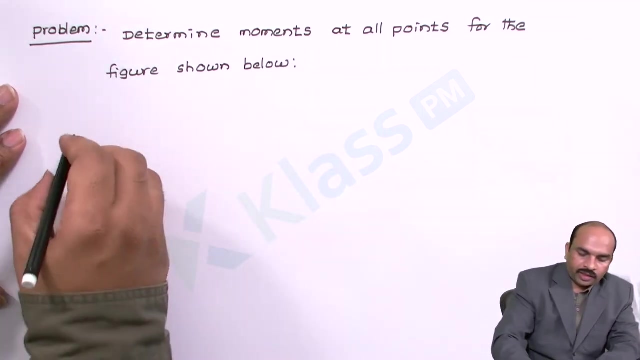 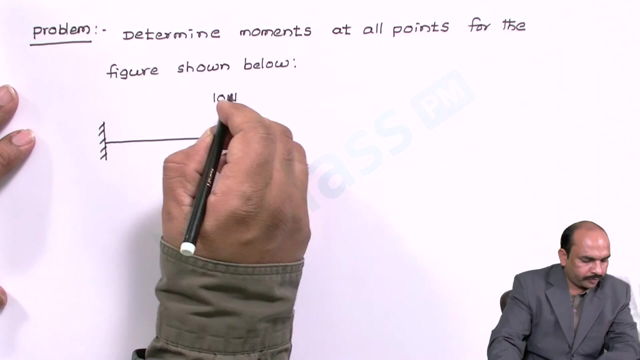 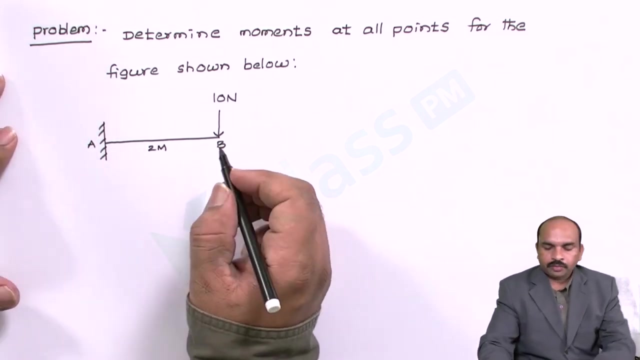 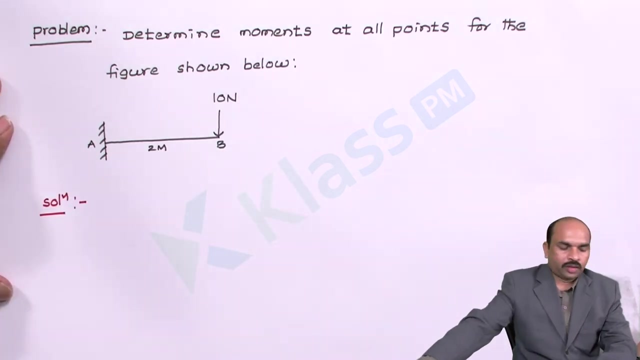 solution is needed to answer your question. The problem is determine moments at all points for the figure shown below. so the given diagram. So this is the given problem: let us calculate moments at all points. let us solve this problem Now. so first let us calculate moment of the force at point A, so we know moment equal. 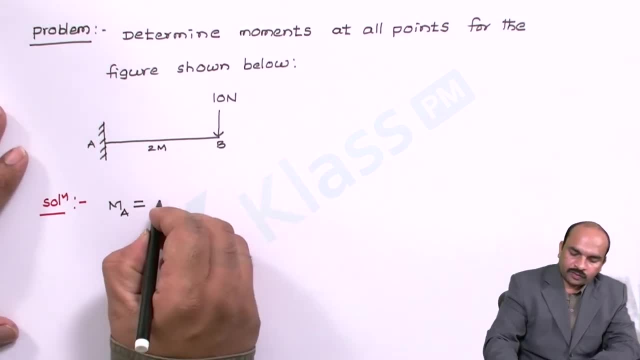 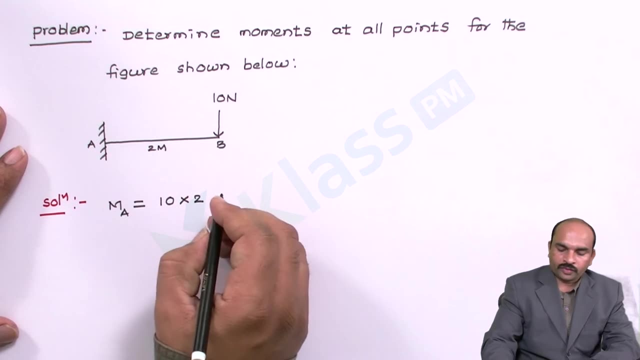 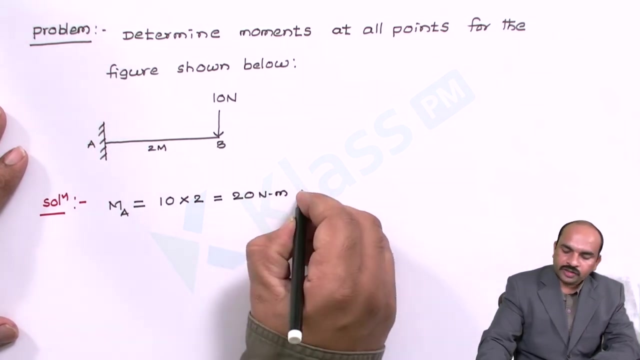 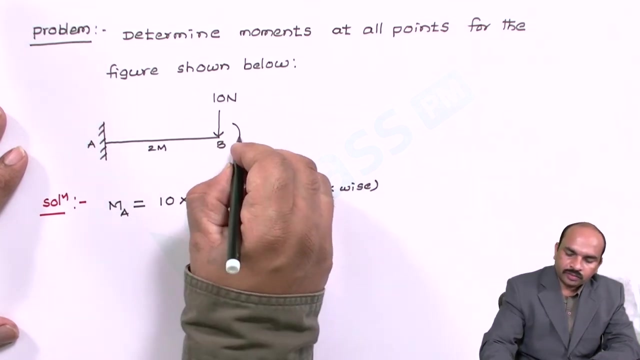 to force into perpendicular distance. so there is a force 10 Newtons into force, 10 Newtons, its perpendicular distance is 2, so 10 into 2, that is 20 Newton meter and it is a clockwise, so it is a clockwise moment. 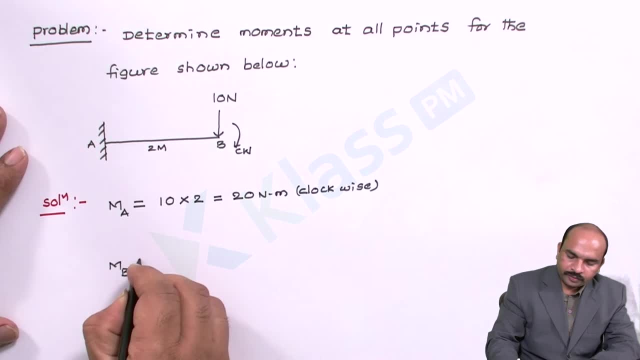 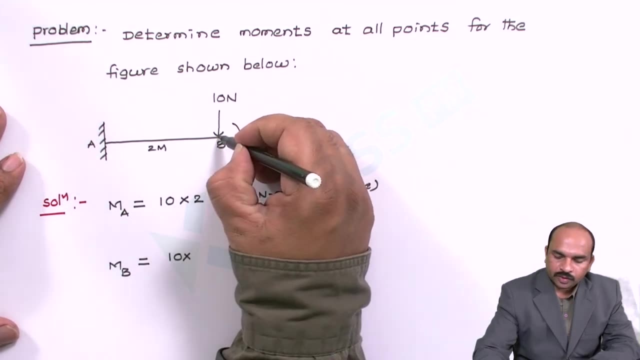 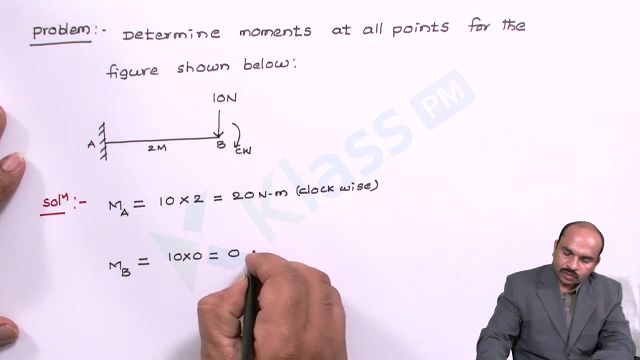 Now, similarly, at point B, the force is 10 Newtons into. the perpendicular distance into this force from B is 0, because the force and point B both are in the same line, their perpendicular distance is 0, so the total moment will be 0 Newton meter. and these are the answers. 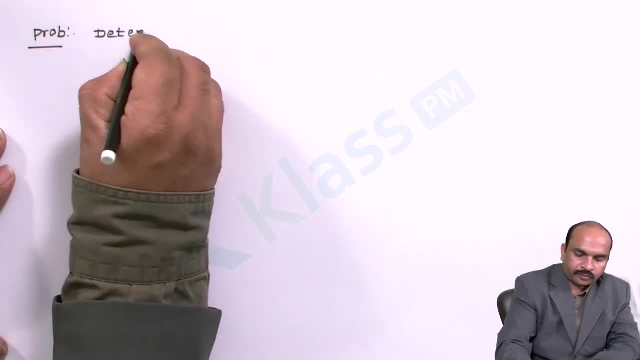 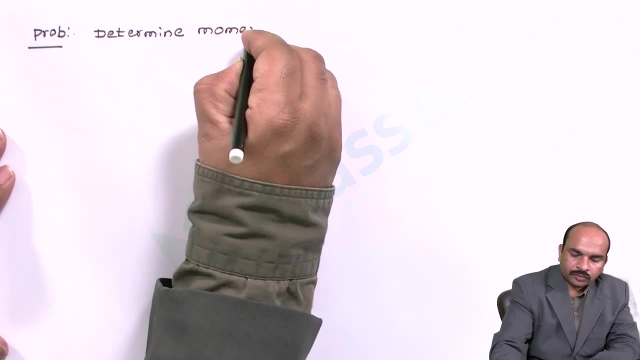 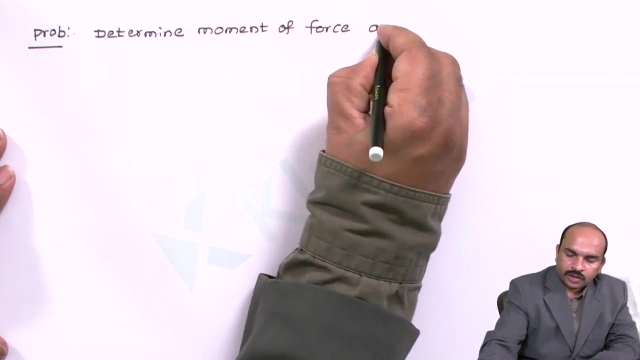 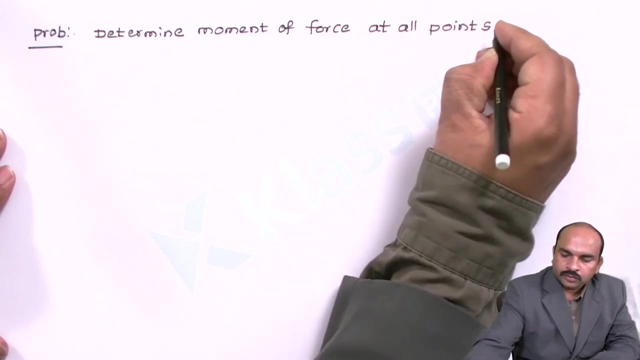 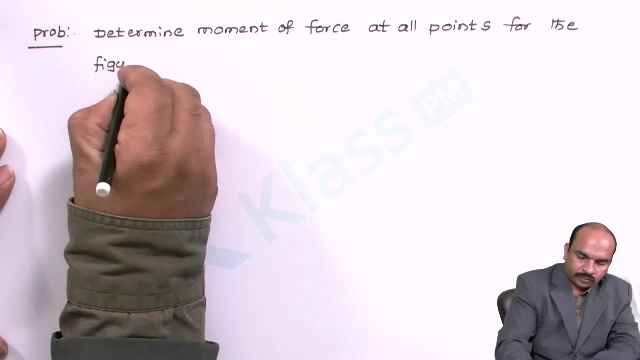 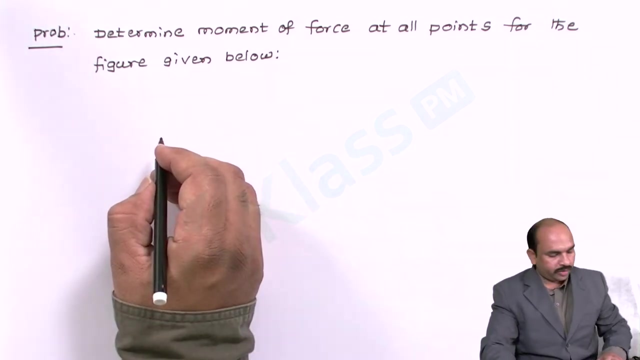 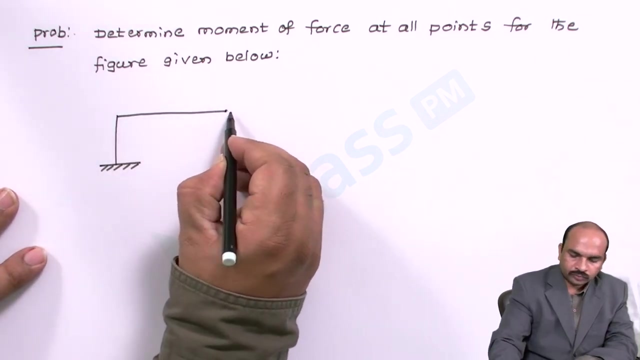 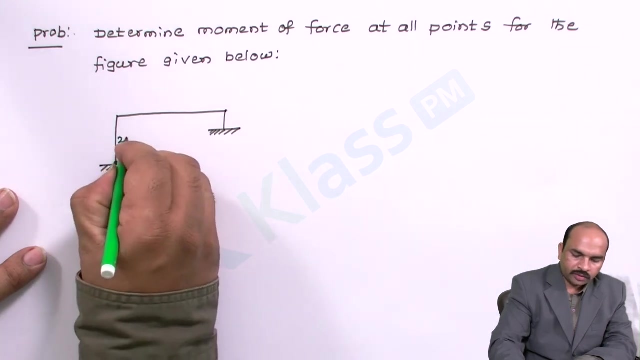 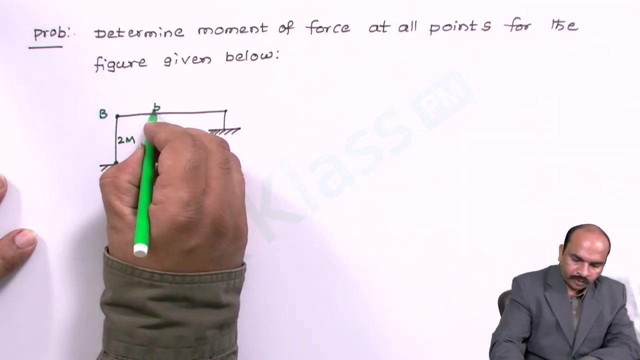 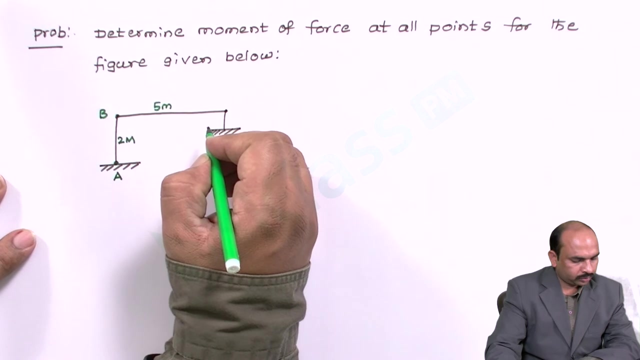 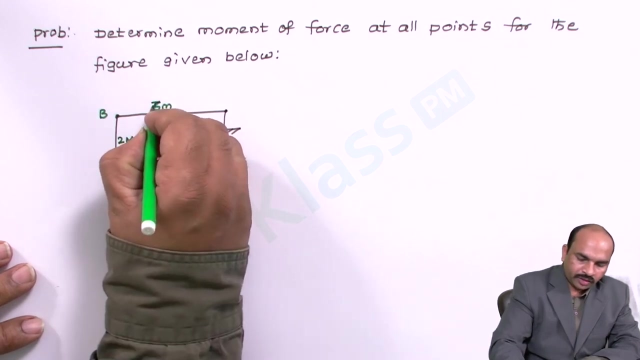 So let us take a look at the problem, determine the moment of force at all points for the figure given below. Now the diagram is given. so this point given as A, this length 2 meter, and this is point B, its length is 5 meter. its length is 2 meter given and its length is 3 meter. 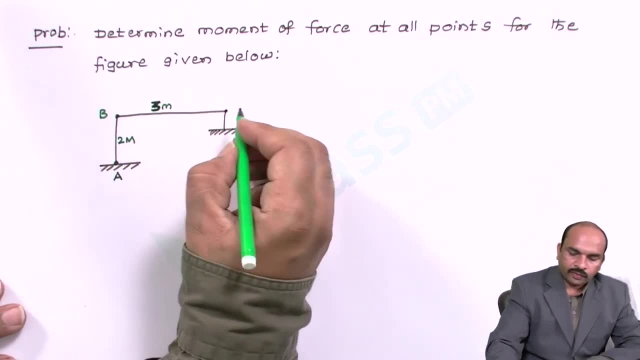 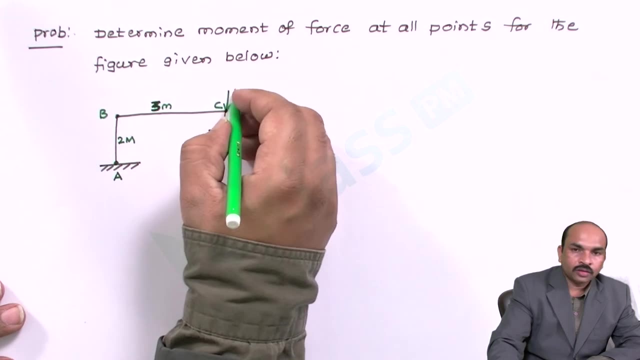 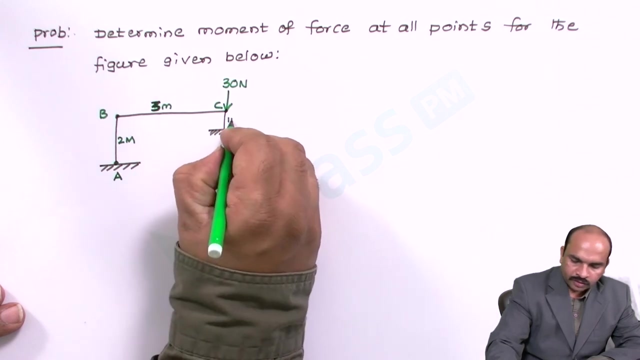 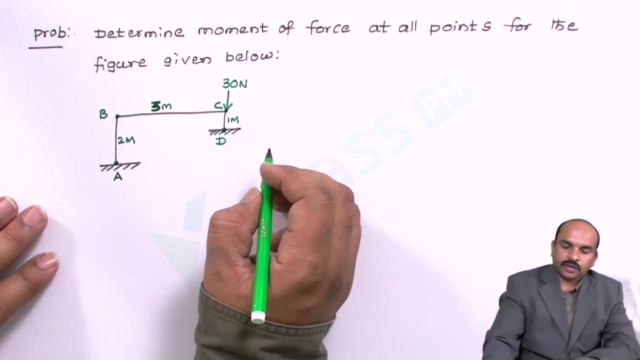 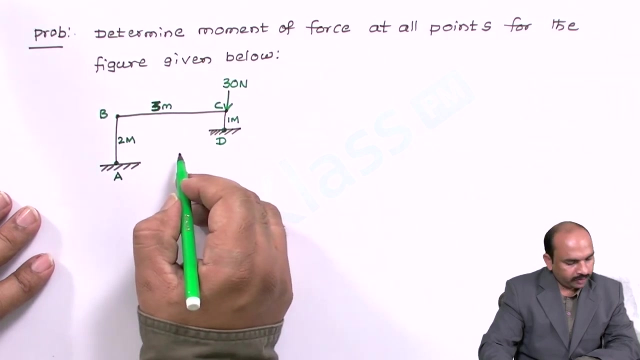 Then there is a force at point C acting vertically downward, and that force is 30 Newtons. Now its length is 1 meter. this point is Now. the question is: he is asking to determine movement of force at all points for the given diatom. 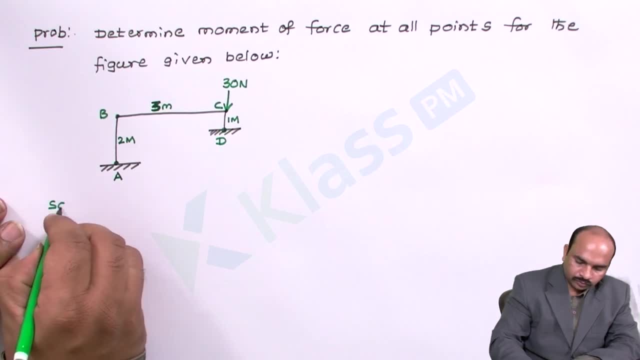 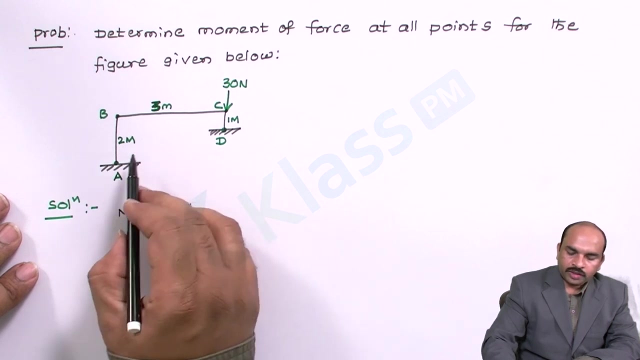 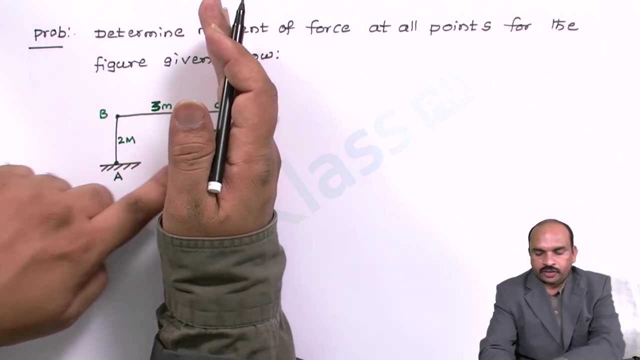 So let us solve this problem Now. first let us calculate movement at point A. Now there is a force, 30 Newton, into its perpendicular distance. Perpendicular distance of this force from this point A, This distance is 3.. So 30 into 3..